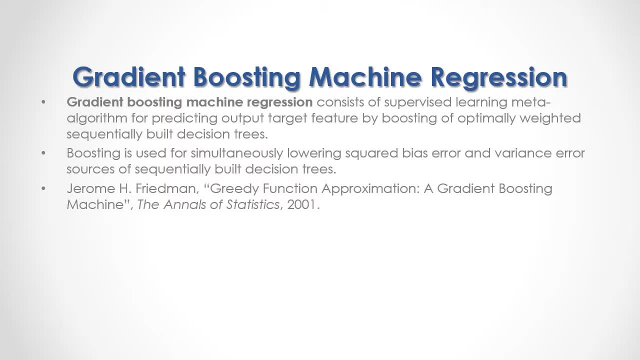 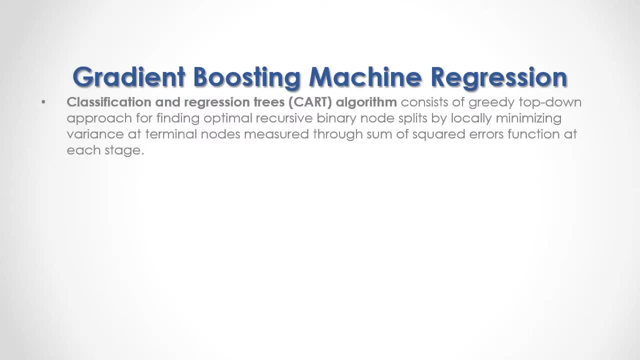 Boosting Machine. It was published in the analysis of statistics in 2001.. Classification and regression trees algorithm consists of greedy top-down approach for finding optimal recursive binary node splits by locally minimizing variance at terminal nodes measured through sum of square errors function at each stage. 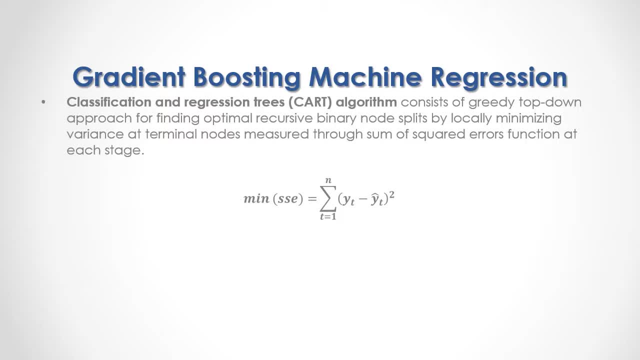 As a formula we have, the minimization of sum of square errors equals to the sum, from the first to the last, Of the difference between outputs: Output target feature data minus terminal node output target feature mean, and that result to the power of 2.. 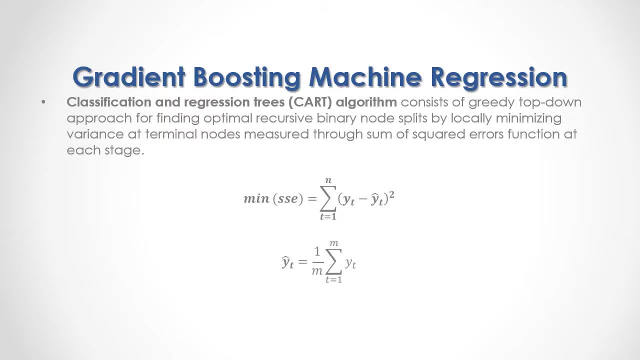 Terminal node output target feature mean in turn is equal to 1 divided by m. m is the number of observations in terminal node multiplied by the sum from the first to the last of the output target feature. data Tree boosting algorithm consists of predicting output target feature of weighted sequentially. 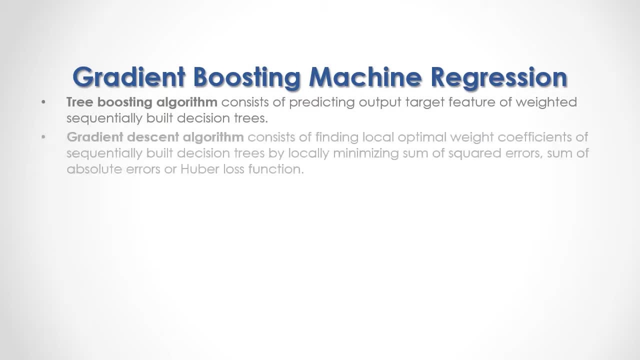 built decision trees. Gradient descent algorithm consists of finding local optimal weight coefficients of sequentially built decision trees by locally minimizing sum of square errors, sum of absolute errors or Huber loss function As a formula. here is an example. we have the minimization of the sum of square errors equals. 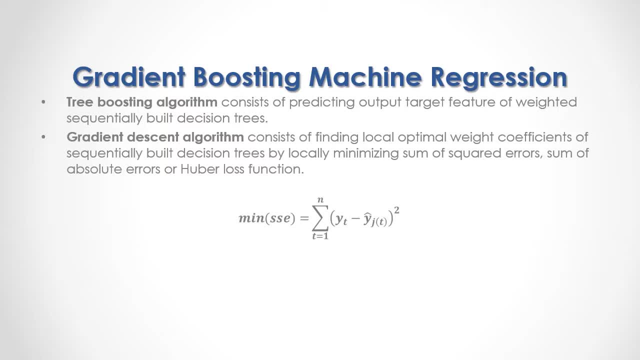 to the sum from the first to the last of the difference between the output target feature data minus terminal node output target feature data. The minimization of sum of square errors equals to sum over the sum of square errors equals to m minus m- sair times m-s. 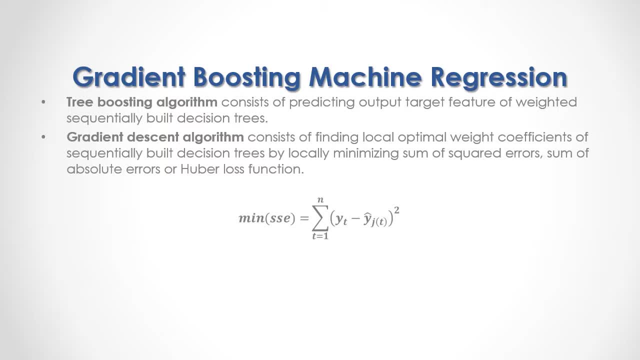 We can also look at the sum of the output target feature data minus terminal node output target feature data. The result of this is subpar. The obediently built decision tree is broad, which means that m is equal to m-s. m is equal. to m-s. m-s-s divided by m-s squared squared squared squared squared squared. Instead, we can do a linear equation in which m-s is equal to m-s squared-squared-squared squared-squared-squared. 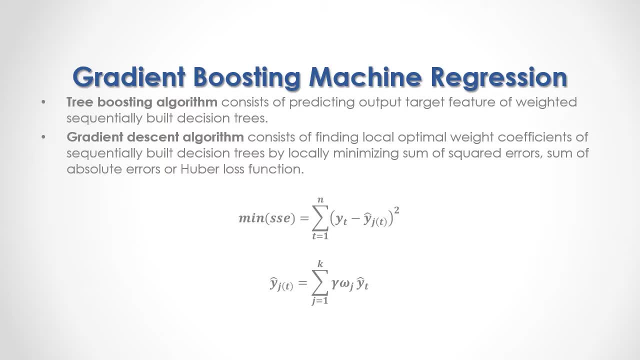 We can use this equation to calculate how to use a linear equation to calculate the weighted output target feature data of a tit-con or t-con. prediction sum in turn is equal to the sum from the first to the last. in this case, k is the number. 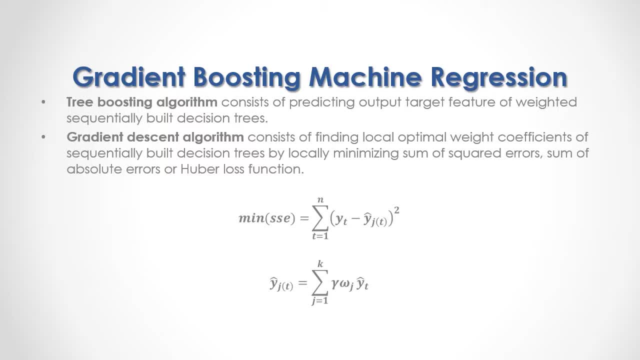 of sequentially built decision trees. and then we have first of all the learning rate regularization coefficient multiplied by the local optimal sequentially built decision trees weight coefficients, and that is multiplied by sequentially built decision trees output target feature prediction- great. so let's go into R studio so that we can study gradient boosting machine. 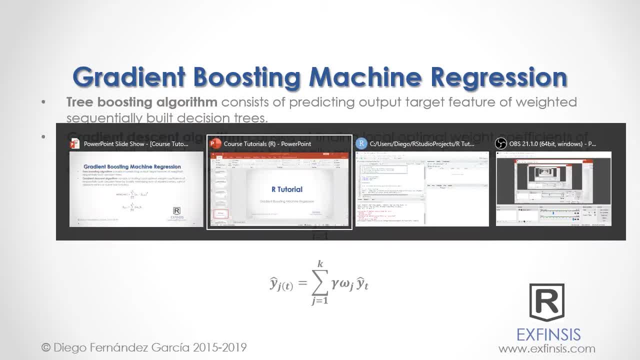 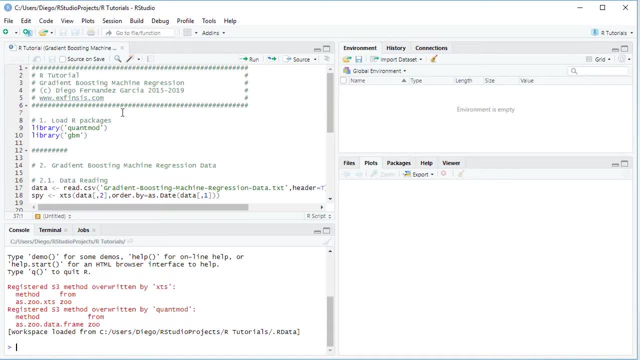 regression with greater detail. excellent. so here we are within R studio. the first step within the tutorial is to load its packages. this is done with the library function and within a dependent function- subheading, as well as a function in the distribution mode, the actual package name. So for this tutorial we'll be using QuadMod and GBM, So we select 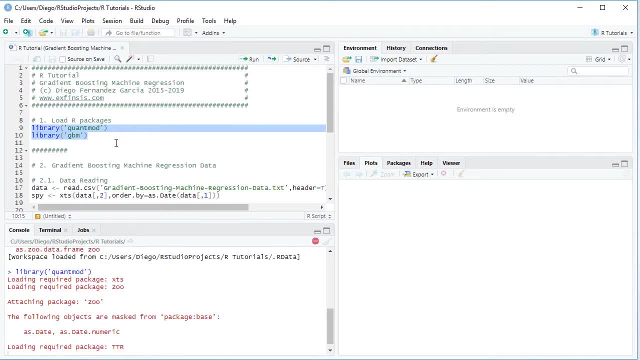 these two code lines, we click run or ctrl enter on the keyboard, which is equivalent. The next step is to create data for the gradient boosting machine regression. This is done through data reading. So we create this variable named data, which is equal to readcsv and within it we have the name of the data. 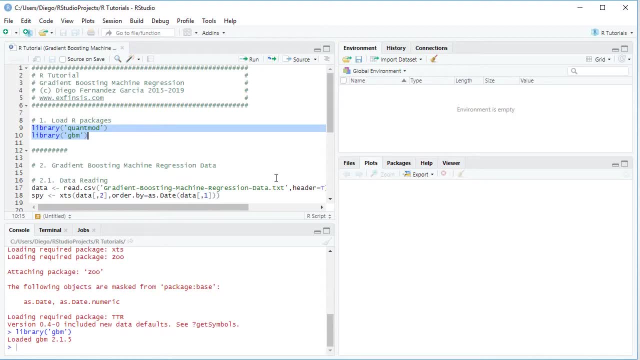 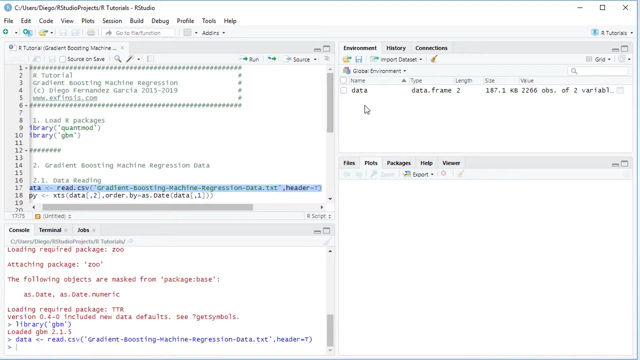 file creating boosting machine regression data as a plain text file with csv or comma separated values stored within the working directory. comma header equals to true, So we select that code line there, click run or ctrl enter on the keyboard, which is equivalent, and that creates the data object within the 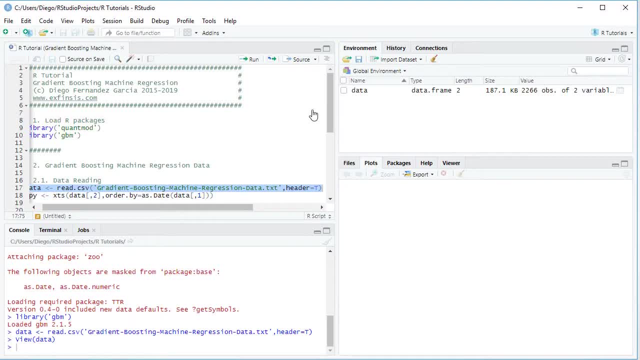 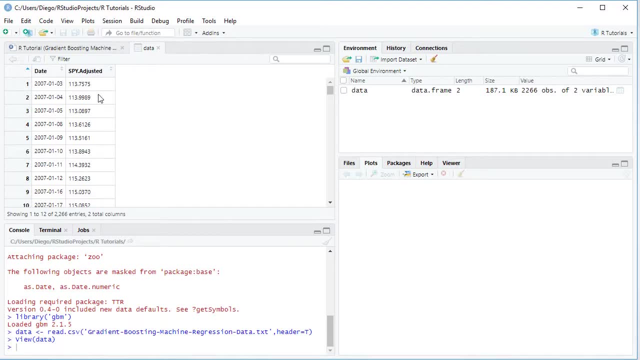 global environment as a data frame. So we click on the spreadsheet kind of icon and it opens the data for us. Within it we have two columns of data: dates and SPF. So we click on the spreadsheet kind of icon and it opens the data for us. Within it we have two columns of data: dates and SPF. 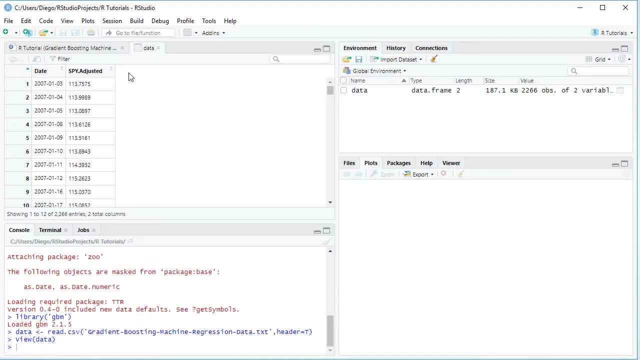 SPY. adjusted SPY corresponds to the ETF investment vehicle which intends to replicate the standard and Poor's 500 index, and adjusted because this includes adjusted close prices, which were adjusted for dividends and splits. And notice: we have data with the daily frequency from the beginning of 2007. 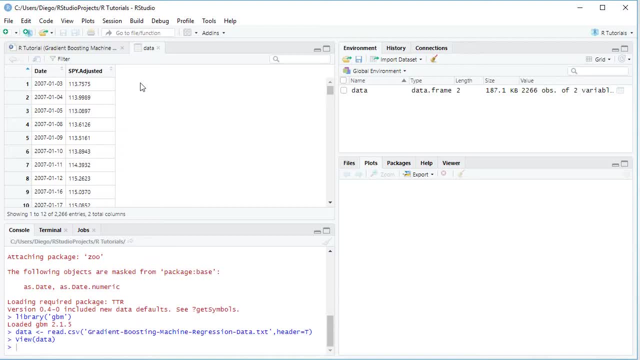 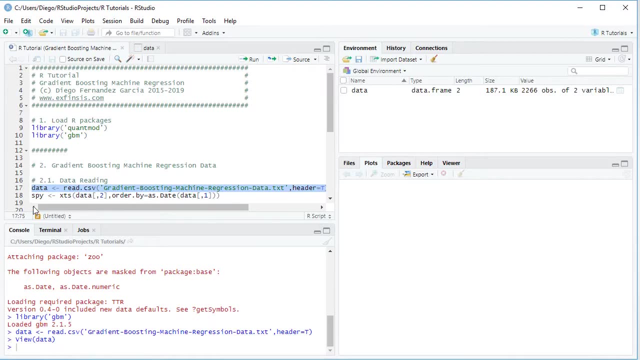 all the way to the end of 2015,. therefore, nine years of data. So back into the code file. The next step is we are going to create an extensible time series which we're going to name SPY. So we can see here, SPY equals to that XTS, or extensible time series, and we're 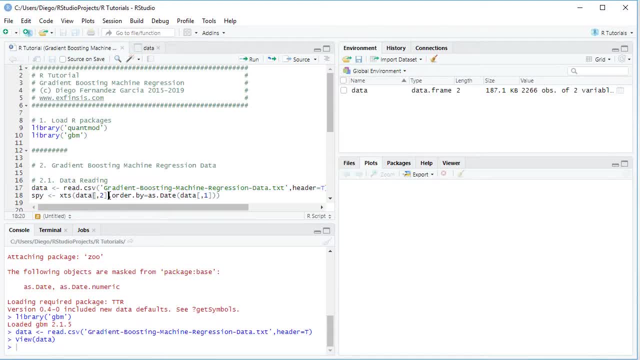 going to select from the previously created data, the second column, the one with the adjusted close prices which were adjusted for dividends and splits order by equals as date with capital D data, the first column, the one with the dates. So we select that code line there and again click run or ctrl enter on the. 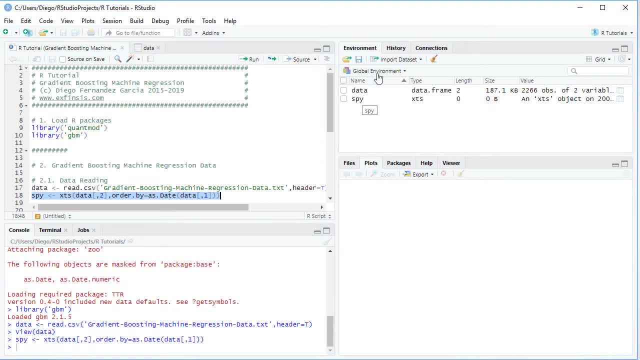 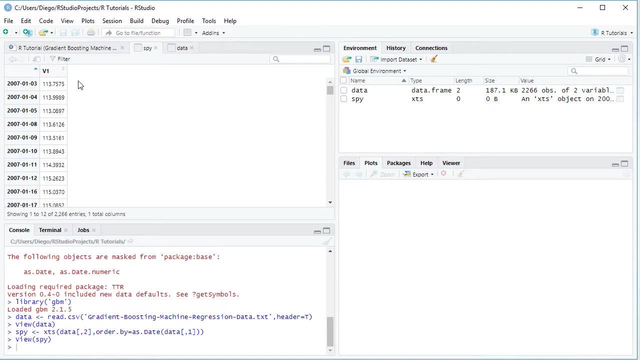 keyboard which is equivalent and that creates an SPY object again within the global environment as an XTS or extensible time series, and we click the spreadsheet kind of icon here and we can see the data object SPY and we have the same data as within data. 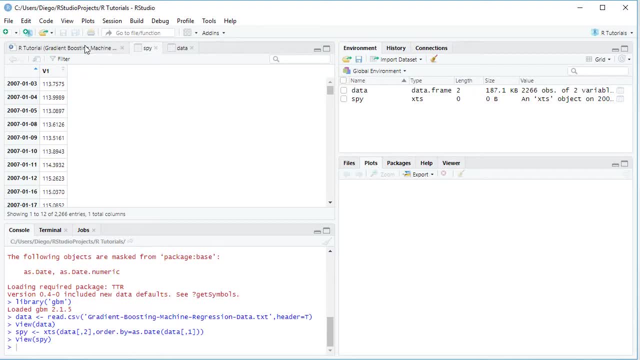 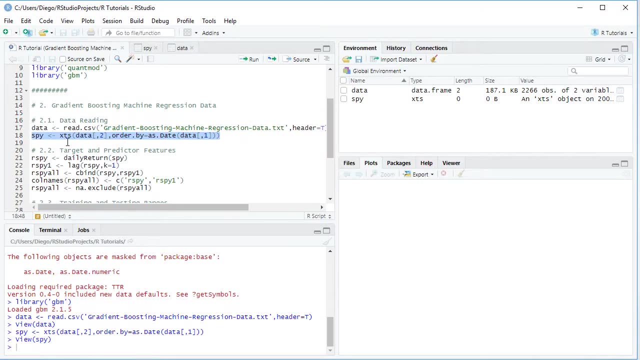 But now the dates became its index soup. so now that we read our data, we're going to continue to create target and predict the features. So first of all, we have a target feature, which is our SPY are, because we're going to calculate its daily arithmetic. greater increases rate. 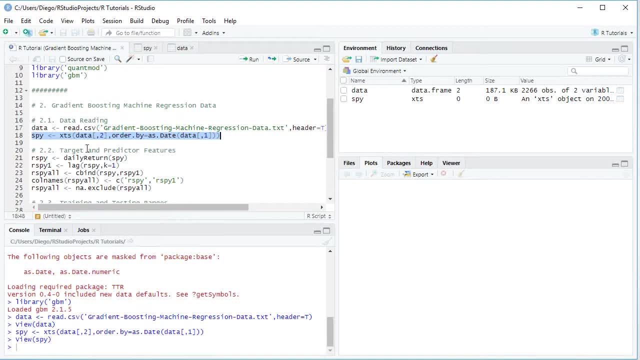 return. So we'll be using daily return function with capital R for SPY. So this is going to calculate, as mentioned previously, the daily arithmetic rate of return of those SPY adjusted close prices which were adjusted for dividends and splits, And then we create the target feature. 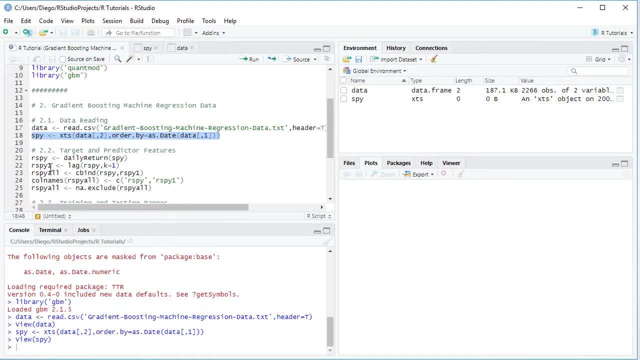 After creating the target feature, we create the predictor feature, which is RSPY1.. So as target feature we have current day returns and as predictor feature we'll be using previous days returns. That's why we use lag here for RSPY and k equals to 1.. We bring both of this together. 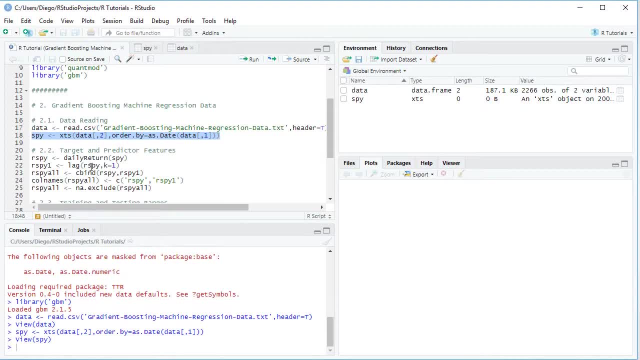 within one data frame, which we're going to name RSPY all, and we bring them together with C bind or column bind in which we have RSPY, the target feature, RSPY1, the predictor feature or current. 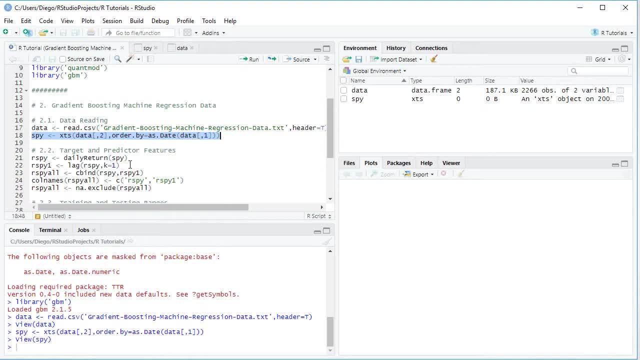 day returns as a target feature and previous days returns as predictor feature. We rename the column names of this variable with the variable names and notice something important here: When we're lagging, we're not using the target feature, We're using the predictor feature, So we're not. 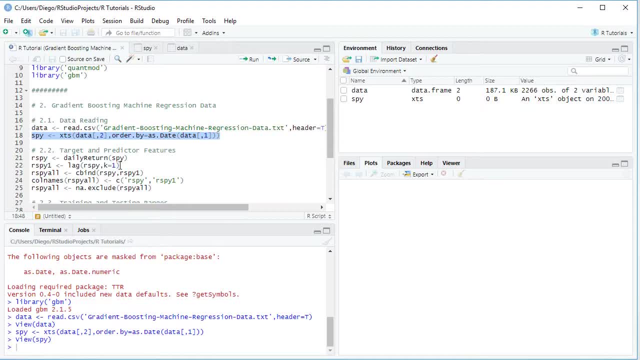 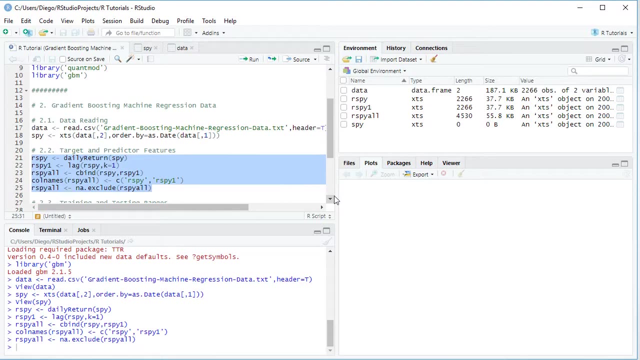 lagging the data. The first observation would be a non-available. so we want to remove that full row of data and we do so with NA, exclude of the previously created RSPY all. So we select all these code lines, click, run or ctrl enter on the keyboard, which is equivalent. The next step is: 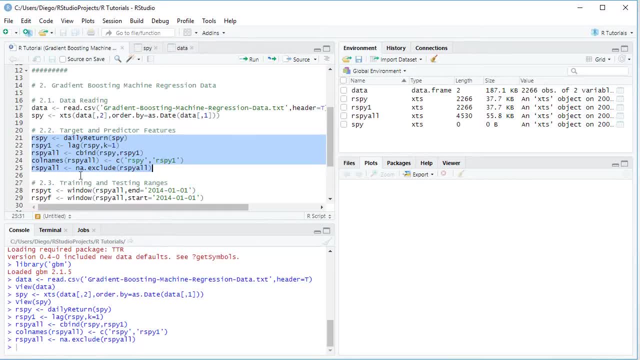 we're going to do our training and testing ranges. delimiting Training range is commonly used for algorithm training and testing range for algorithm testing to evaluate forecasting accuracy. So we create first of all training range- RSPYT T- for training range- and then testing. 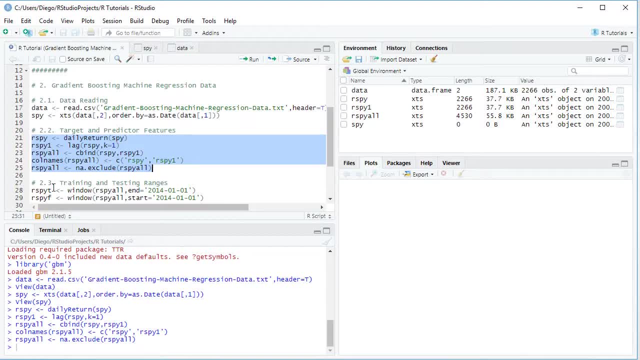 range, RSPYFF, to distinguish it from the training range, And in both cases we'll be using window function. so the corresponding training range is going to be from RSPY. all We're going to select from the beginning of time series, which is 2007,. and it's going to end at the beginning of 2014.. So 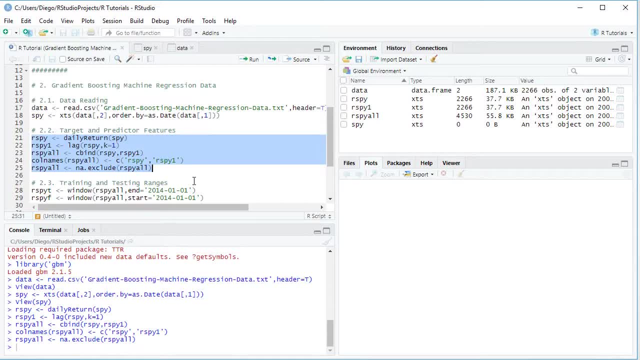 we'll be using the first seven years of data as our training range And for the testing range again from RSPY. all we're going to select from the beginning. that's why we have start at the beginning of 2014, all the way to the end of 2015,. 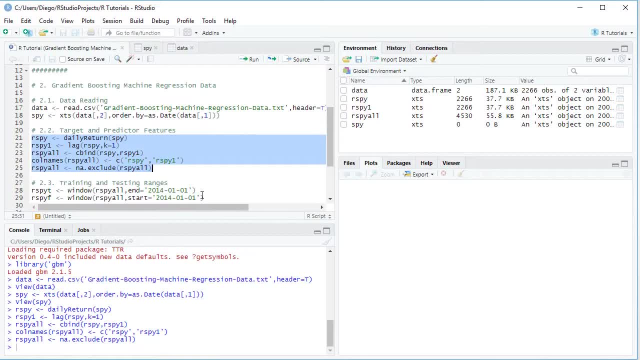 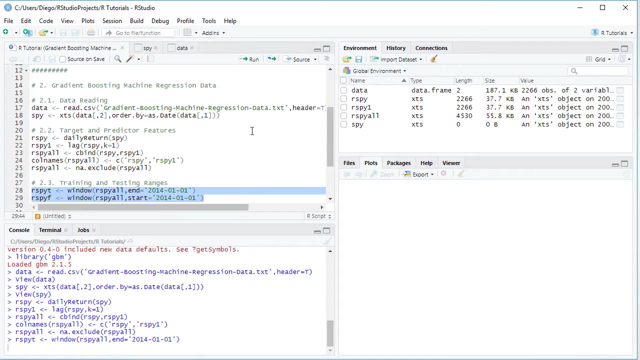 therefore the last two years of data as a testing range. Notice that this training and testing range delimiting was only clear, for educational purposes. therefore it is not fixed and it can be modified according to your needs. So we're going to select these two code lines: click run or ctrl enter on. 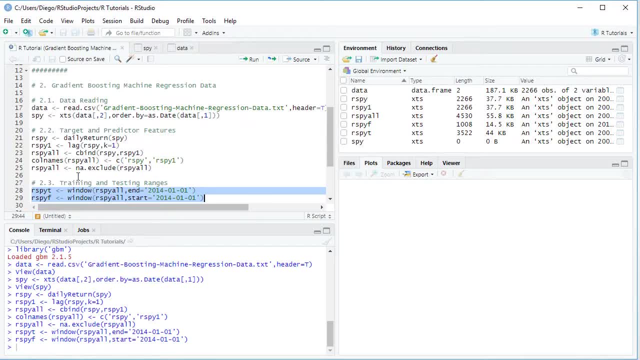 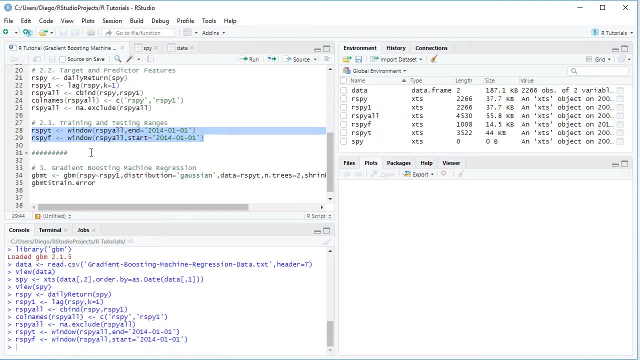 the keyboard and notice that within this tutorial, we'll only be working within the training range. So now that we have our data ready and the delimiting of training and testing ranges, we're going to continue with gradient boosting machine regression. So here we have the creation. 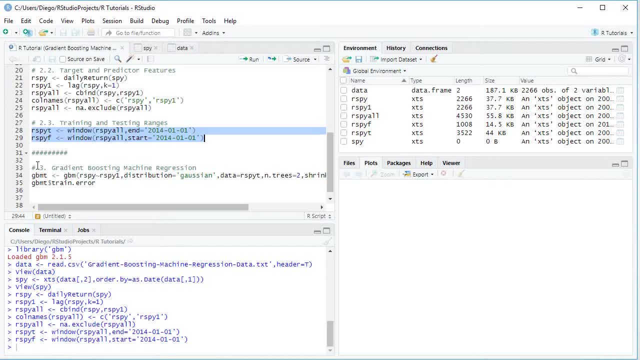 of this corresponding object, which is the gradient boosting machine, or GBM, and notice that we included T because this is done within the training range And we'll be using GBM function- and first of all, we have the formula which describes the corresponding regression, in which: 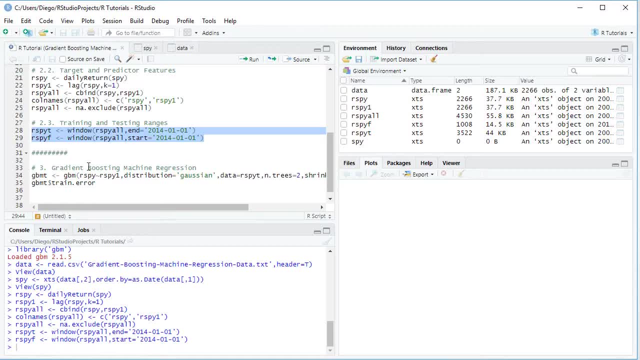 we have the gradient boosting machine and the gradient boosting machine and the gradient boosting machine and we have the target feature RSPY, or current day returns, being explained by RSPY1, which is the predicted feature, or previous days returns. So here we have. distribution equals to: 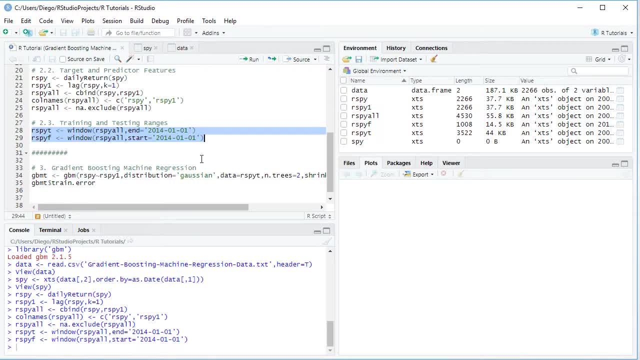 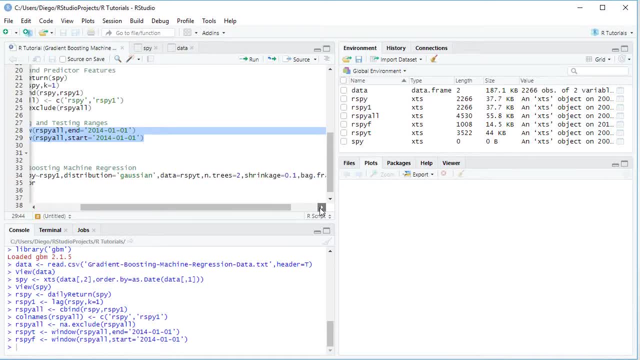 and it's going to be. number of trees: two. Then we have shrinkage equals to 0.1, that's the corresponding learning rate regularization coefficient. and here we have back fraction equals to one, so that's the training range fraction used for model fit. so we're going to be: 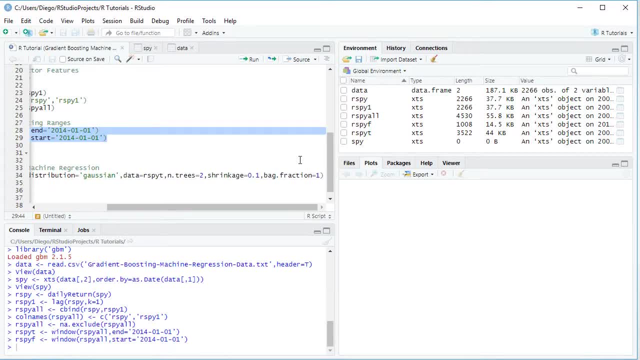 using the full training range for the model fit when doing those sequentially built decision trees. Very important observation regarding these parameters is that they were only included, again for educational purposes, as an example. therefore, they are not fixed and can be modified according to your needs. And then we're going to print from this previously created GBMT its train error. 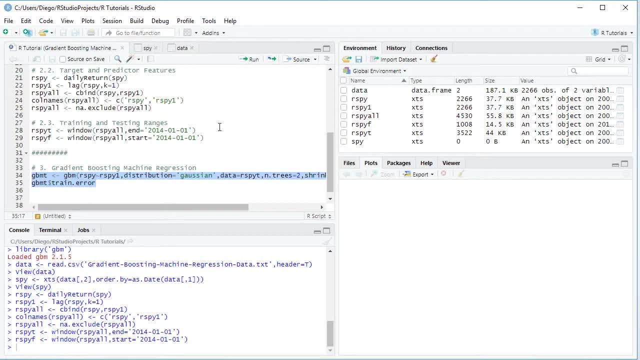 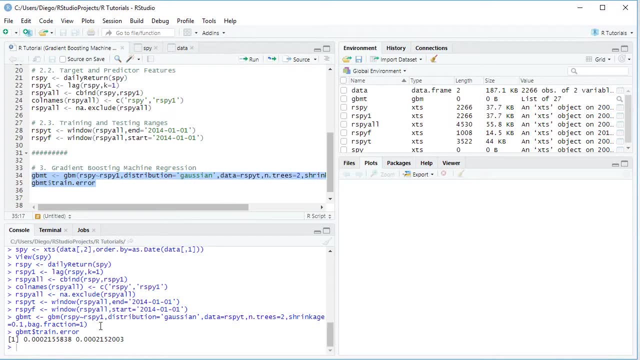 so we're going to select these two code lines here and then we're going to click run or concentrate on the keyboard, which is equivalent, And notice here that it printed the corresponding training error. So, as we can see here we have. 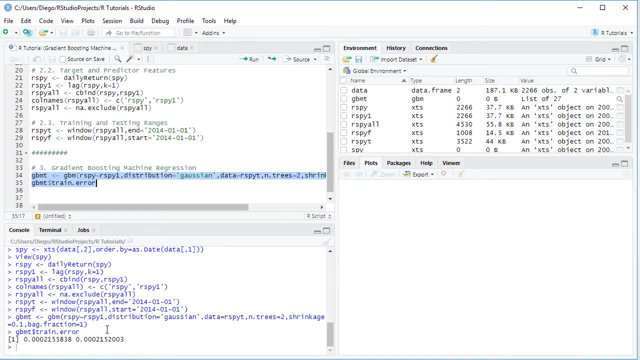 with just one tree and then with the second sequentially built decision tree. so here is when it built the first tree and then the sequentially built second tree and, as we can see that as the number of sequentially built decision trees increased, the corresponding train error in this. 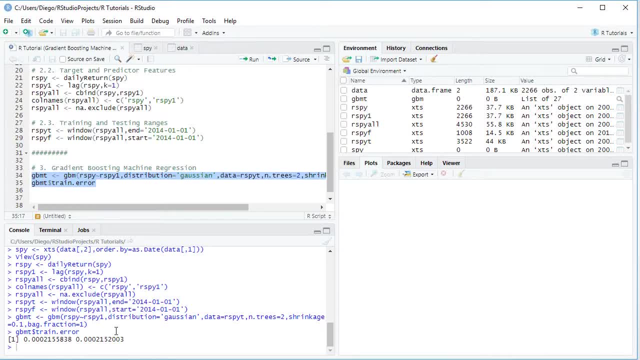 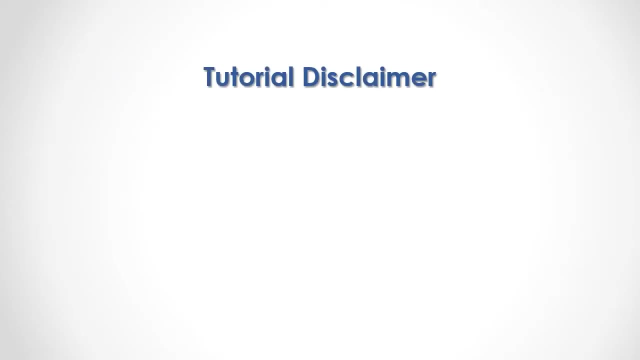 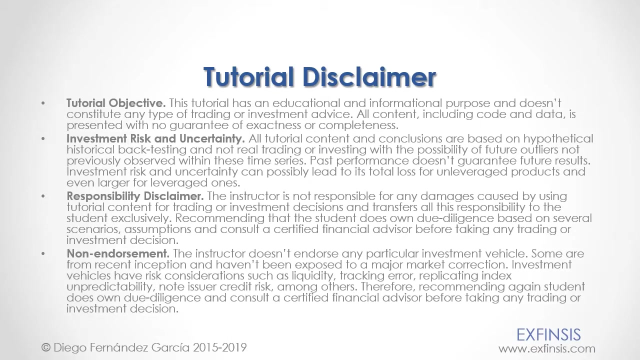 specific example, decreased, Excellent. So now that we finished studying gradient boosting machine regression, let's go back into the slides. And, as mentioned previously, this tutorial has an educational and informational purpose and doesn't constitute any type of trading or investment advice. Please pause the video now so you can.